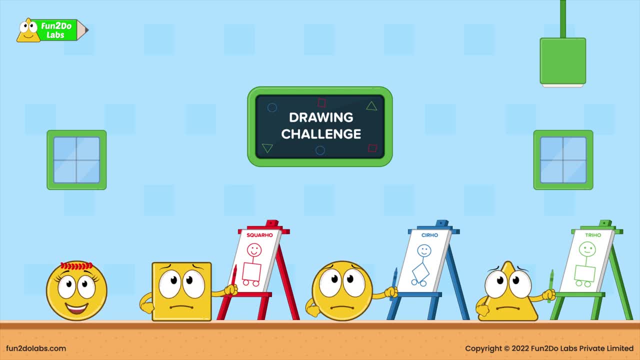 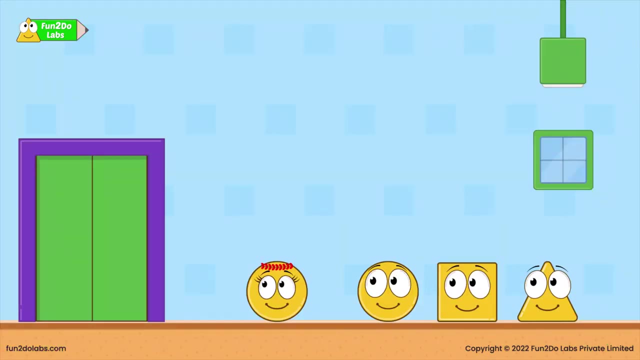 I instructed you to draw a square body. A square has four sides. All your squares have four sides, But why do they look different? How should I decide the winner now? Who could it be? Ah, It is Uncle Math at the door. He is here to give a box to Square-O. 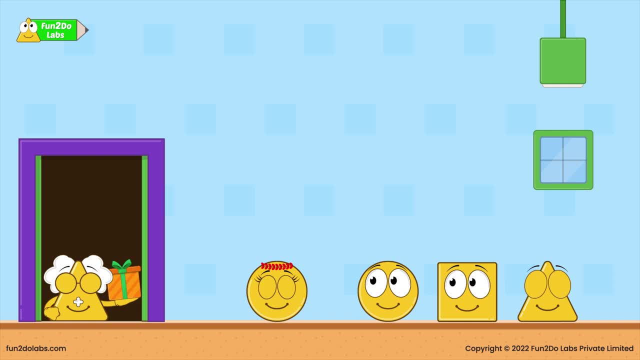 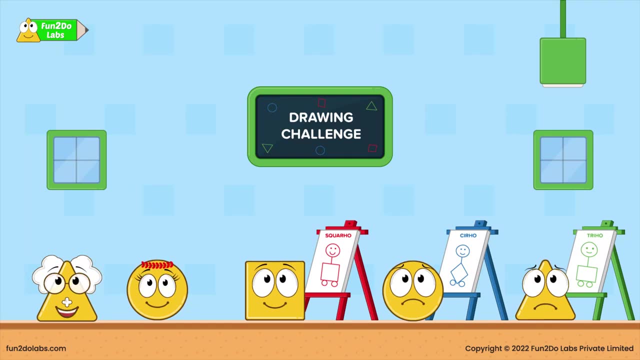 Sirha is happy to see Uncle Math and request him to come inside to help her decide the winner. Clearly, Square-O is the winner, Sirha, But why are we not the winners? We also drew squares. Yes, our squares look different. 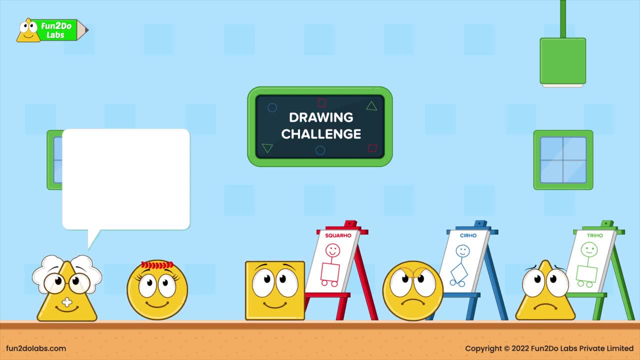 But they are squares at the end of the day. Right, Children? you remembered that a square has four sides, But you forgot one important thing about squares: All the sides of a square are equal. Sriho, see, Two of your sides are short and two are long. 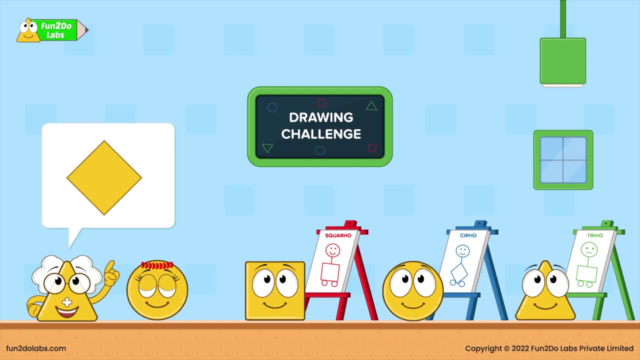 You drew a rectangle, Sirho, you drew a diamond shape. A diamond shape is a square that is pulled from its corners. The diamond shape looks like a kite. Sriho and Sirho understand their mistakes. So Square-O drew a square. 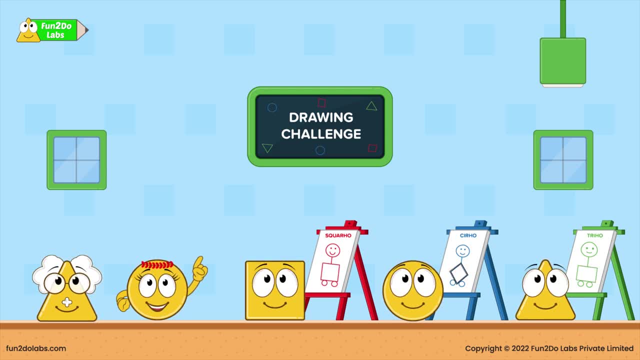 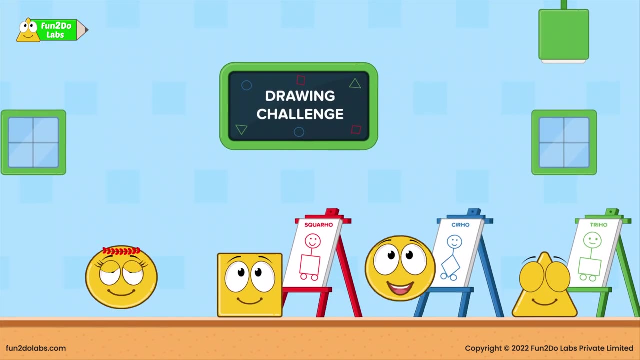 Sriho drew a rectangle and Sirho drew a diamond. Clearly, Square-O wins. The challenge is over and Uncle Math leaves The kids stay back and play more games. Challenges are fun, but confusions are even more fun. They not only help us gain clarity. 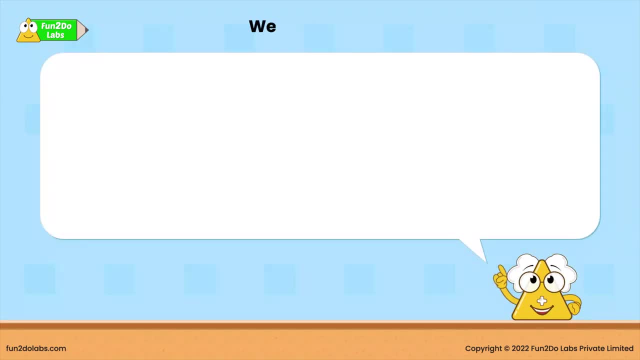 but also help in learning deeply. We learned that a square, a rectangle and a diamond shape all have four sides. All the sides of the square are equal. A rectangle has two short sides and two long sides. A diamond shape is like a square pulled from its corners. 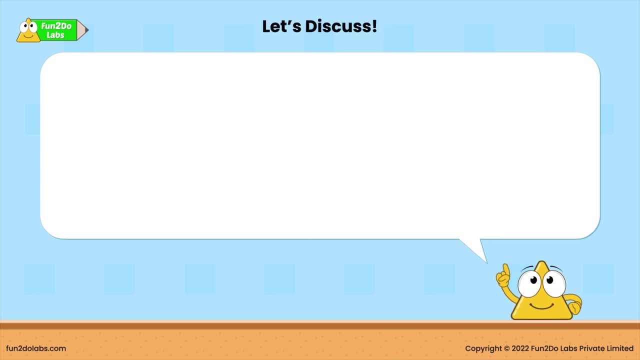 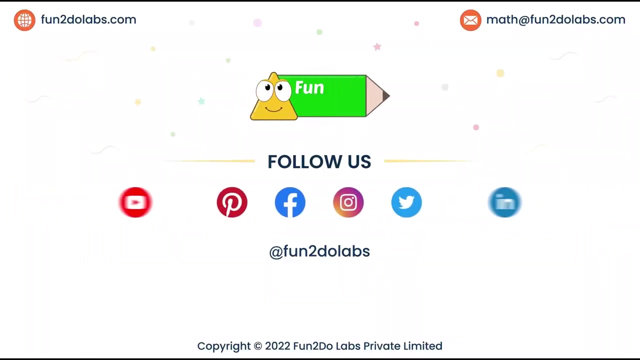 It looks like a kite. Let's discuss What were the rules of Sirho's drawing challenge. Can you explain the difference between square, rectangle and diamond shapes? Confusions help us gain clarity and learn deeply. Do you agree? Follow us on fun to do labs, to enjoy watching more such math stories. songs and games.